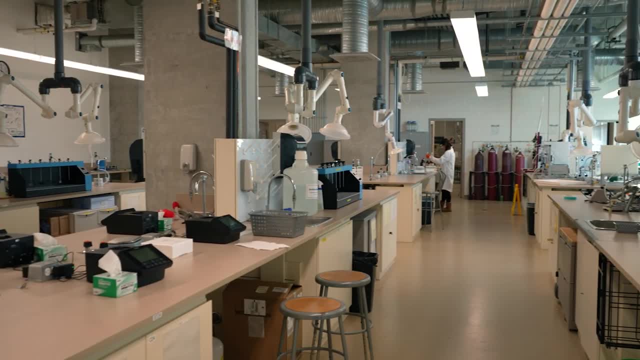 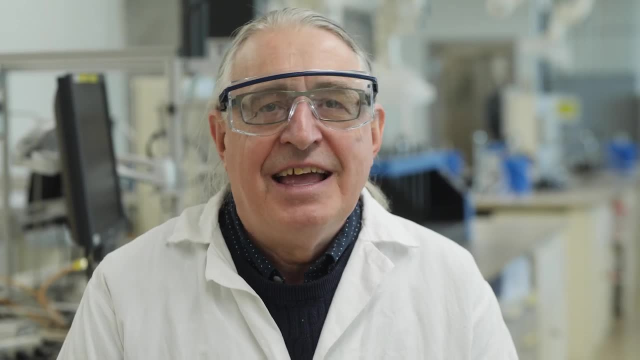 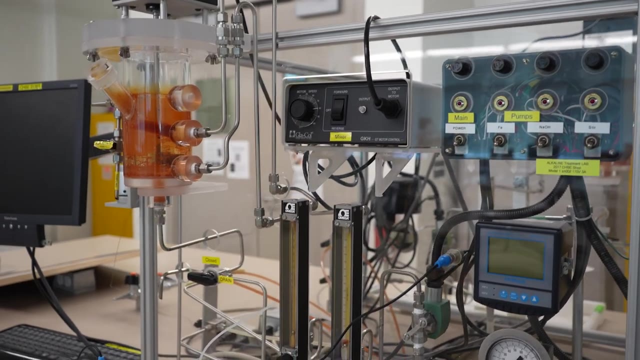 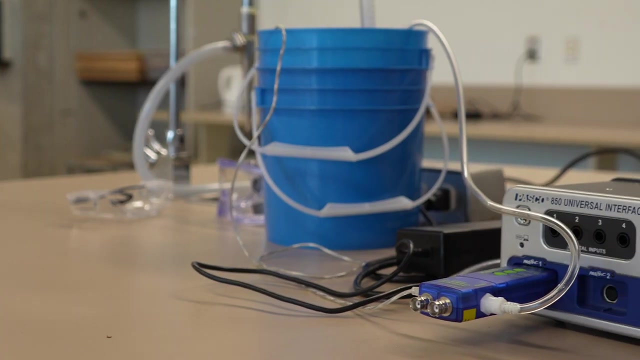 third year environmental engineering student at UBC. The environmental engineering program is basically a combination of those courses within civil engineering and within chemical and biological engineering That focus on environmental issues and topics. My name is Greg Lawrence. I'm a professor in the department of civil engineering here at UBC and my specialty is in the field of environmental fluid. 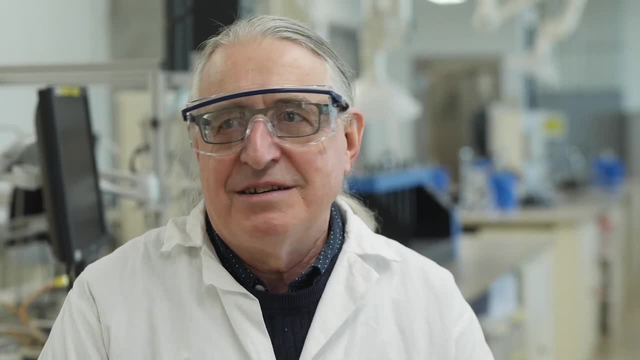 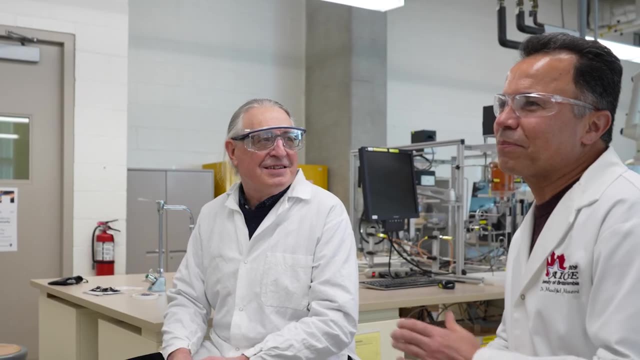 mechanics and, together with Majid, I'm one of the co-directors in this program. My name is Majid Mohseni. I'm a professor here at the department of chemical and biological engineering. Many of our society's challenges have to do something with the environment. 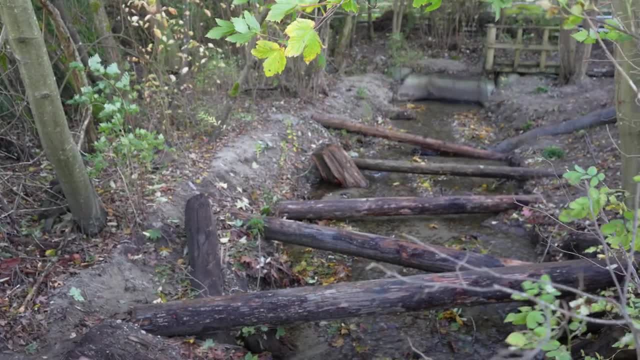 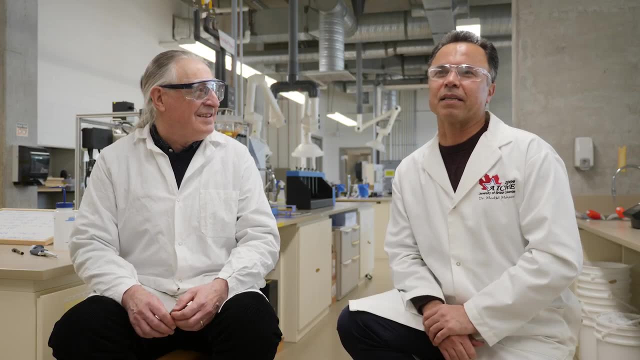 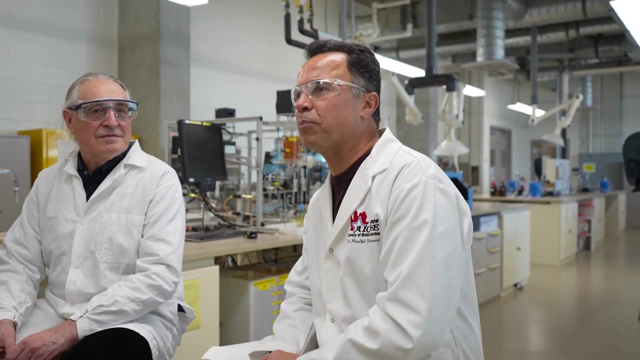 Whether it's climate change, whether it's clean water and sanitation, whether it's air quality. So those require skill sets that our environmental engineers have. Now, of course, our students will have the opportunity to go through the co-op programs. Many of those employers of the co-op 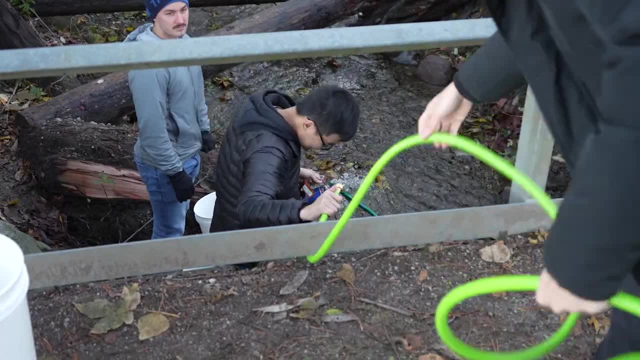 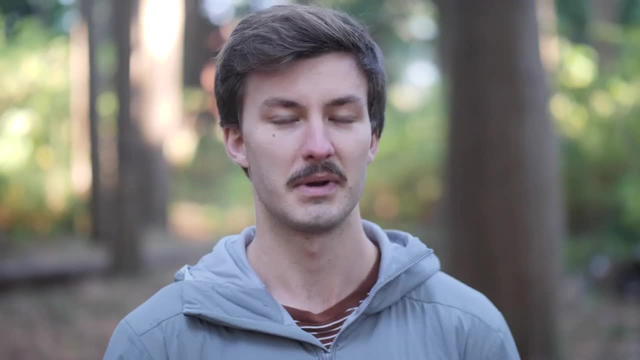 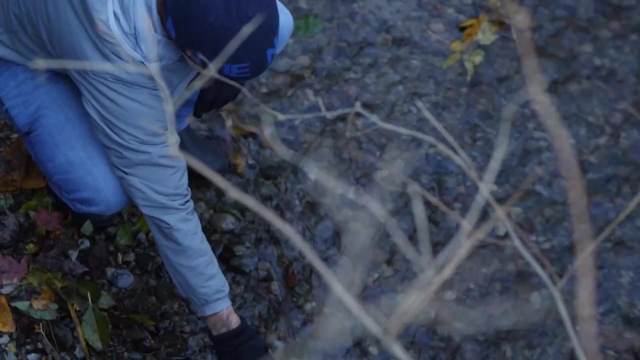 students are also the ones that are part of the advisory group for our program, So the relationship is embedded within the program. My name is Ben and I'm a third year environmental engineering student. For my co-op I worked with Environment and Climate Change Canada measuring the flow rates. 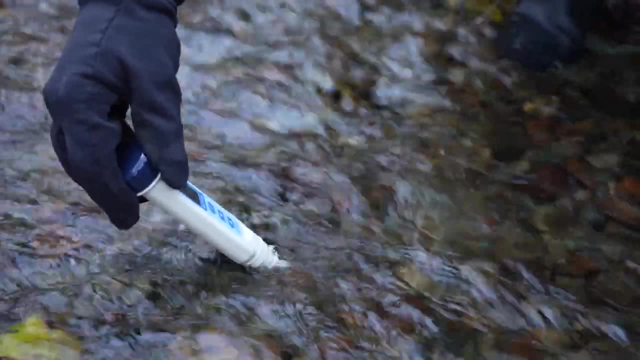 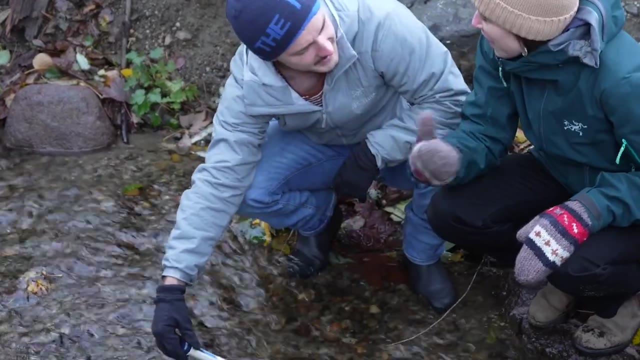 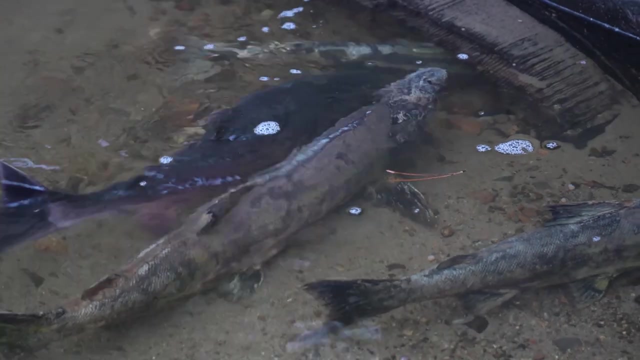 of rivers during the 2021 November floods in BC, which was very exciting. So I got to go to both Merritt and Princeton and do some field work to try to determine what the flow rates were of the rivers. that helped informed decision makers on what they should do during the floods. That really gave me a good opportunity. 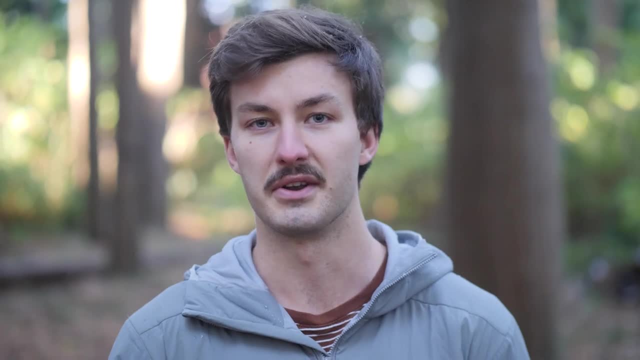 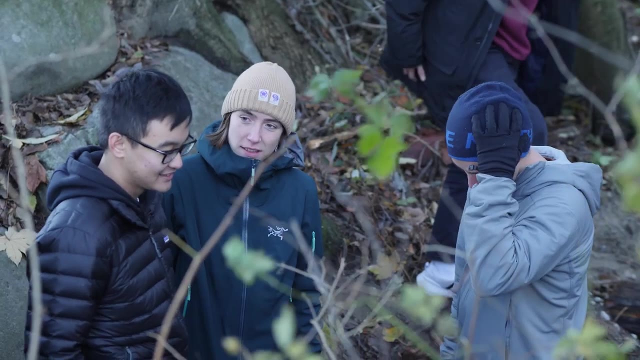 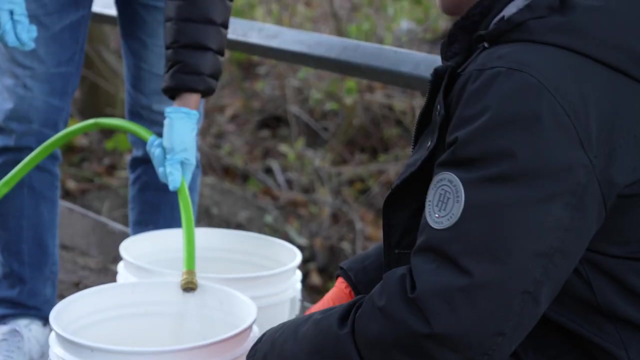 to kind of expand my field work skills and apply a lot of the knowledge I had learned in school. I'm Abby Taylor. I'm in my third year of environmental engineering here at UBC. Last year I worked with a drone reforestation company doing kind of plant science experiments and 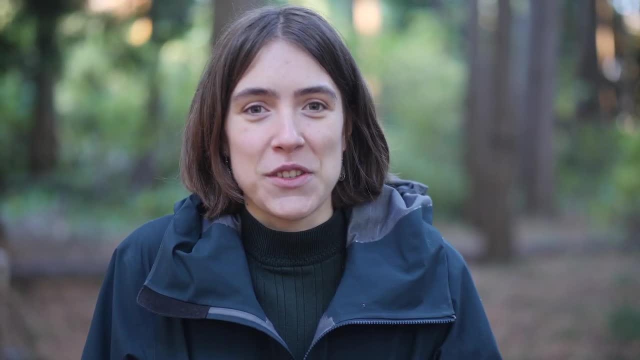 field work as well involved with that. I think it's super important to focus on things like that that can be scaled and can have a big impact in terms of carbon emissions and carbon sequestration. There are small, big, small issues with carbon emissions and carbon sequestration. There are small, big, few issues with carbon emissions and carbon sequestration.